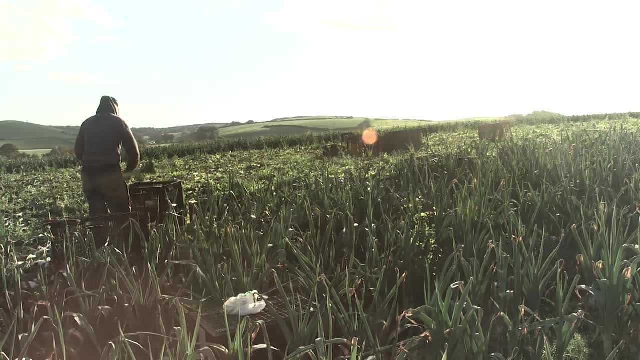 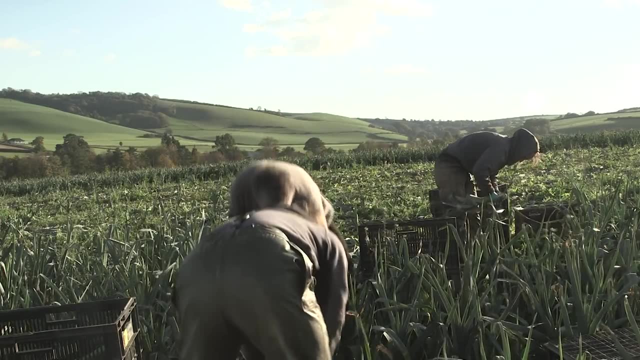 listen to them. We have subsequently found out that there are varieties of leeks which have quite good resistance to rust. by growing those varieties and growing them just a little bit further apart, it really is not necessary to spray leeks with fungicide. I mean, today, I think it's. 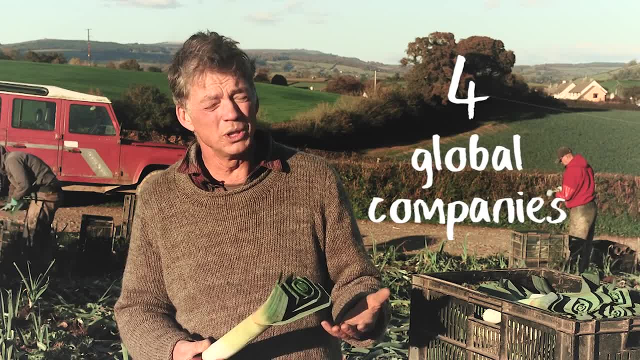 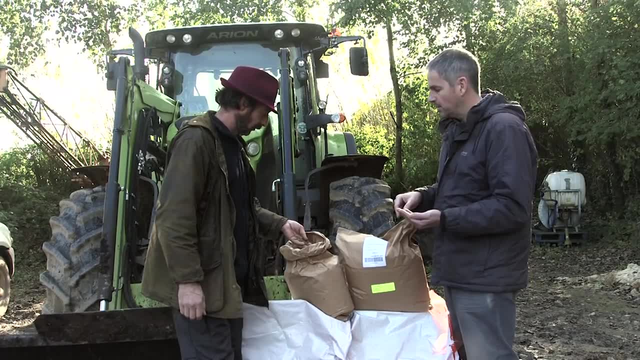 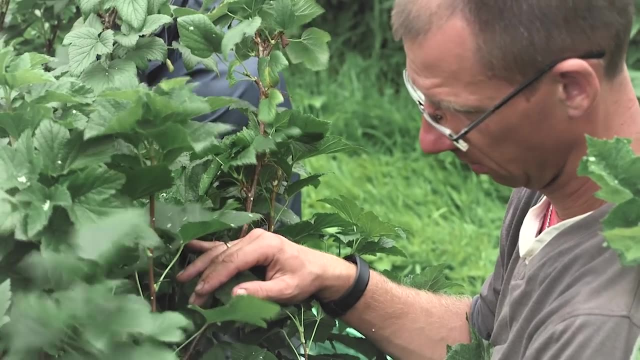 about 75 percent of agrochemicals are sold by four global companies and increasingly, actually, they have also bought up all the seed industry. so you know, they control the supply of seeds and they control the use of chemicals and they have been completely dictating the direction that agriculture. 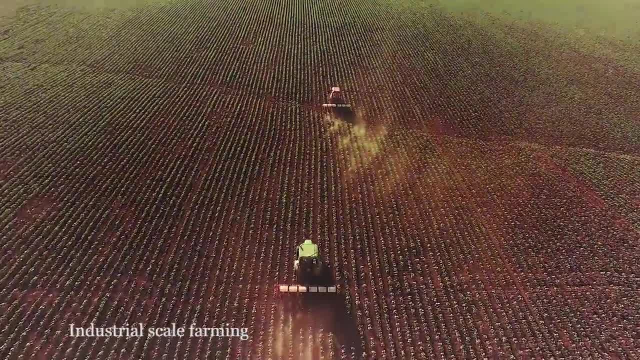 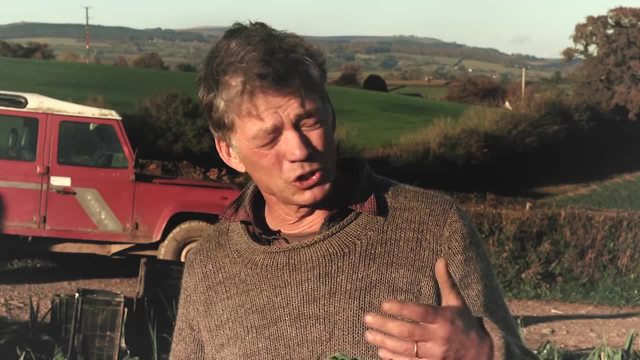 has gone in which is really more about their profits than it is about producing healthy food or maintaining farmers incomes. I mean, I think greenhouses are a really interesting example of what can be done with an ecological, biological approach to pest control. I mean, when we put up 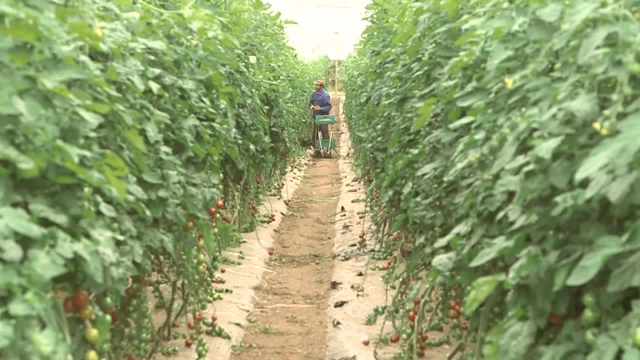 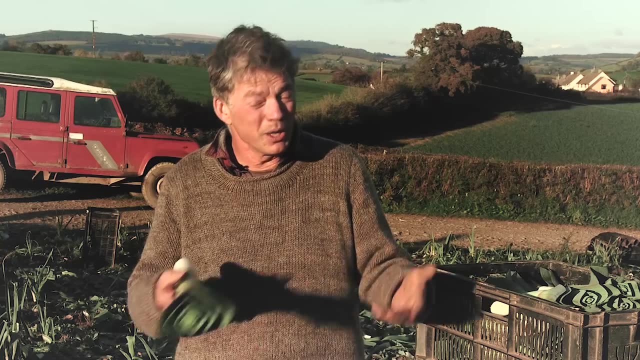 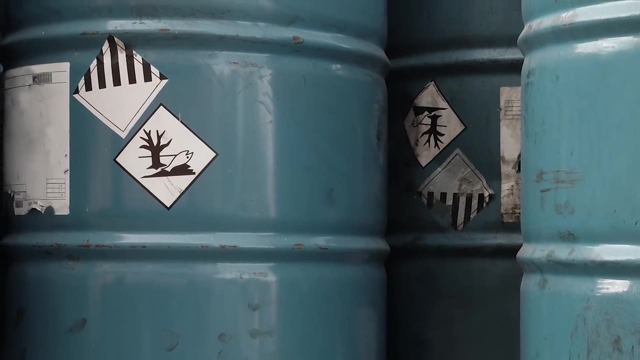 our first tunnels 20 years ago to grow peppers and tomatoes and aubergines for our boxes. they were devastated by red spider, mite and aphids. they just went in there and had a field day and we were then advised to actually fumigate our greenhouses with some really, really toxic chemicals. At the time we 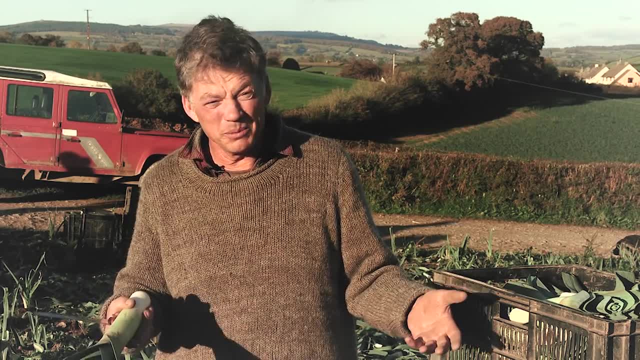 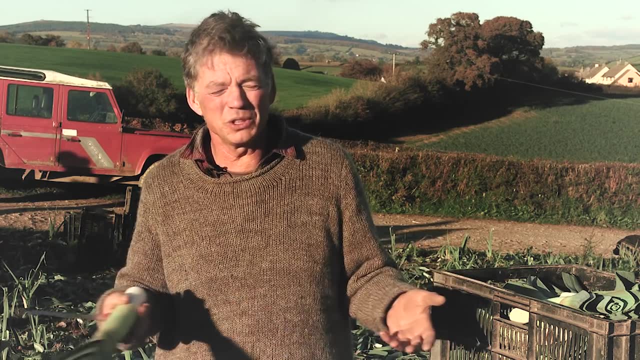 were told that we were safe to use and we were assured by the government that these were safe chemicals to use. I mean, if they were safe then and they're not safe now, I mean, how are we supposed to believe the government when they tell us that it's safe to use neonicotinoids? I mean, you know, I'm 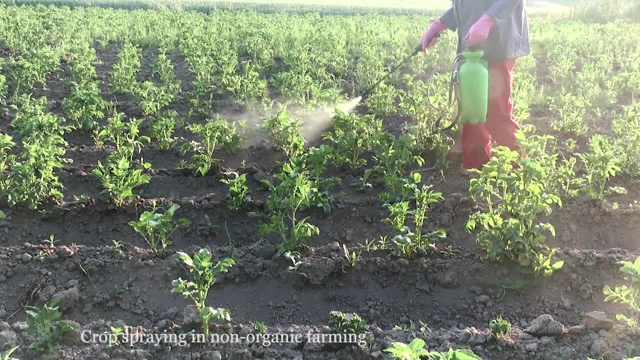 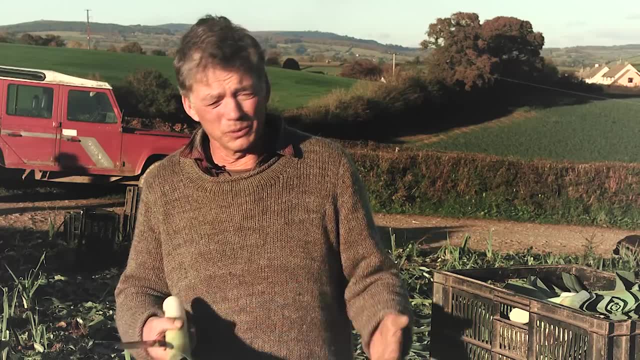 pretty sure that they will be banned, just like virtually all the chemicals that I used as a teenager have been banned. There is no safe level for a nervous system disrupting insecticide. there's no safe level for a hormone disrupting herbicide. I mean, not for a bee. 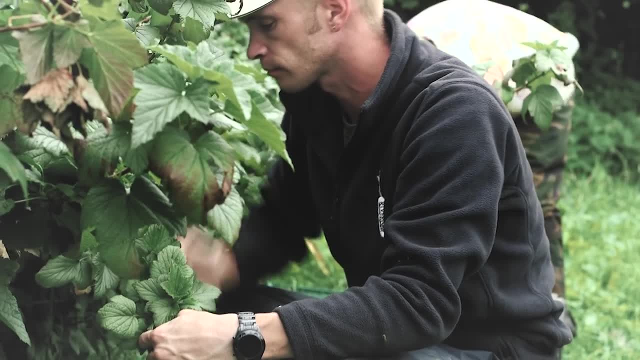 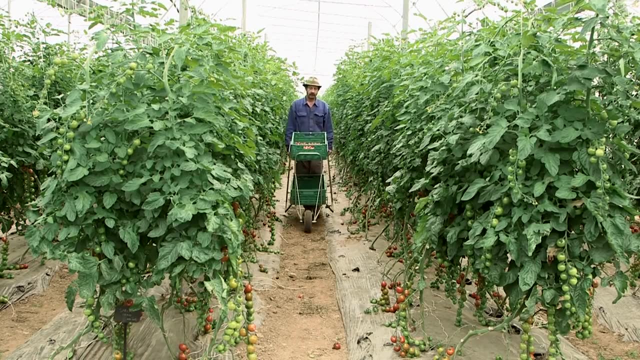 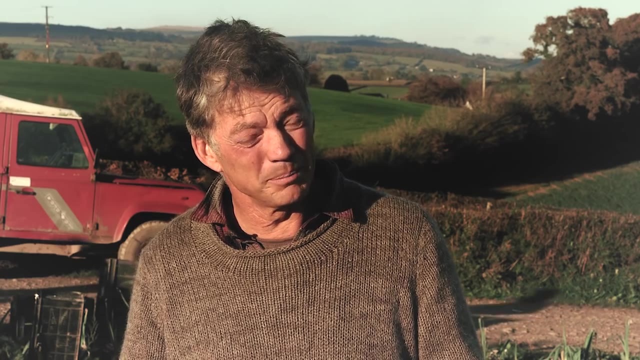 a leek and not for a human. We slowly found that by managing the habitat to encourage the predatory insects, and indeed sometimes actually introducing predatory insects, that we could control all those pests. Interestingly, 20 years later that's what everyone's doing, because all the chemicals they 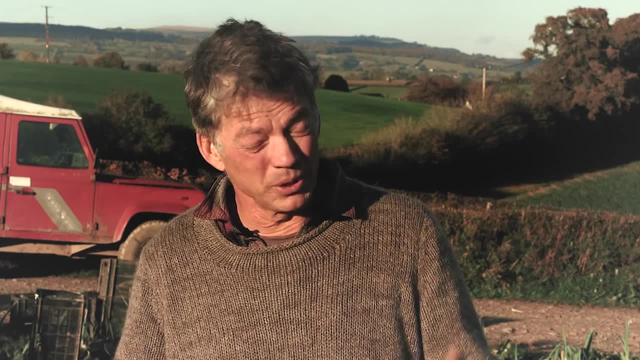 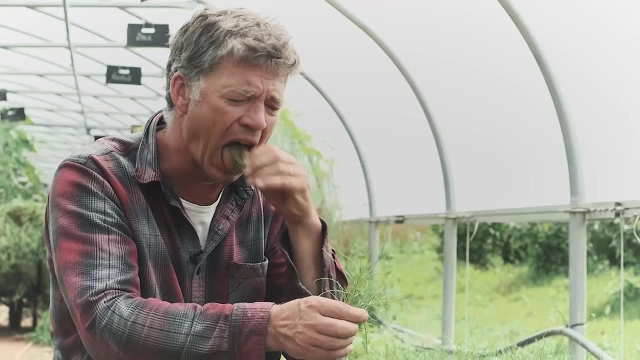 were using. either the insects have acquired resistance because they breed really, really quickly inside a tunnel, or indeed they've been banned because they're not safe for use. So almost everyone is now using neonicotinoids. I mean we've got a lot of people who are using an ecological approach to insect control in greenhouses.